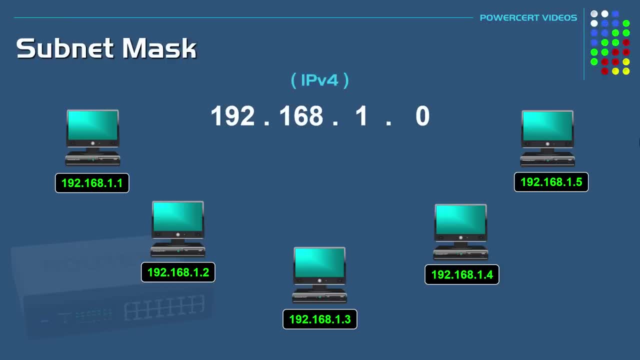 purposes And, to be specific, I'm talking about an IP version 4 address. An IP version 4 address is a 32-bit numeric address written as four numbers separated by periods. Each group of numbers that are separated by periods is called an octet. The number range in each octet is from 0 to 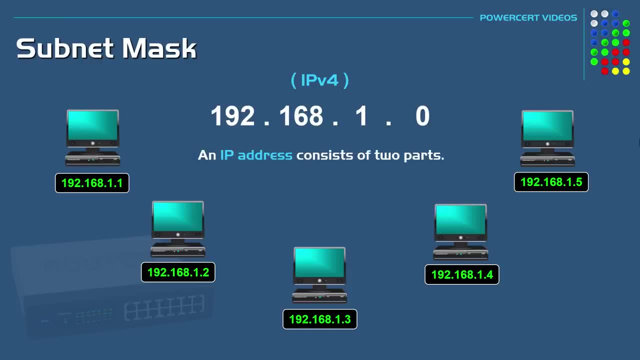 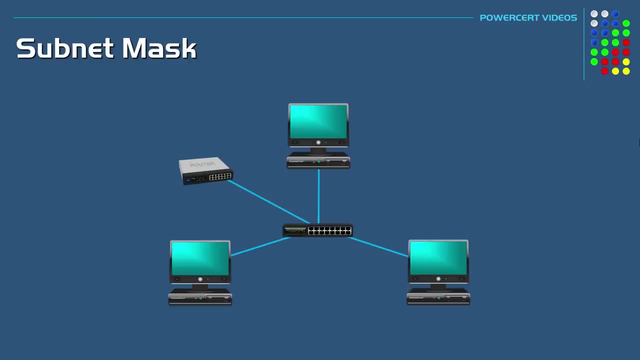 255.. An IP address consists of two parts. The first part is the network address and the second part is the host address. The network address or network ID is a number that's assigned to a network, So every network will have a network address or network ID. The network address or network ID is a 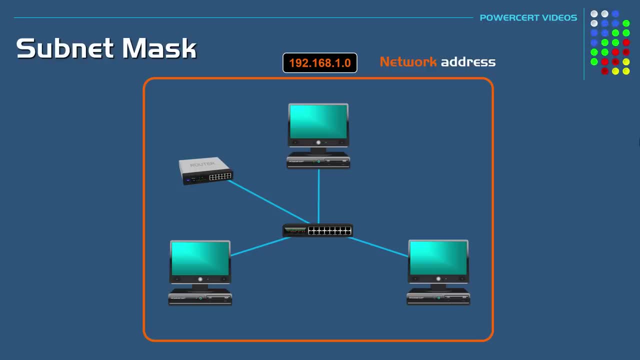 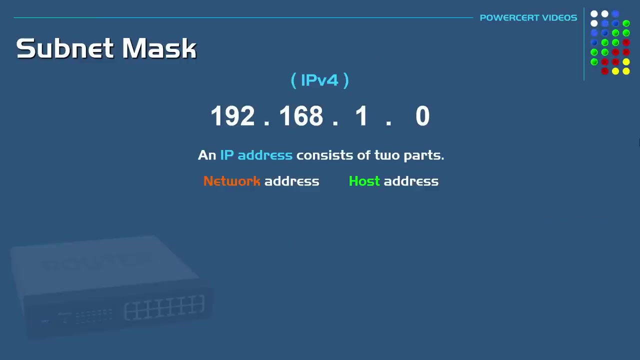 unique address. The host address or host ID is what's assigned to hosts within that network, such as computers, servers, tablets, routers and so on. So every host will have a unique host address. Now the way to tell which portion of the IP address is a network or the host is where the 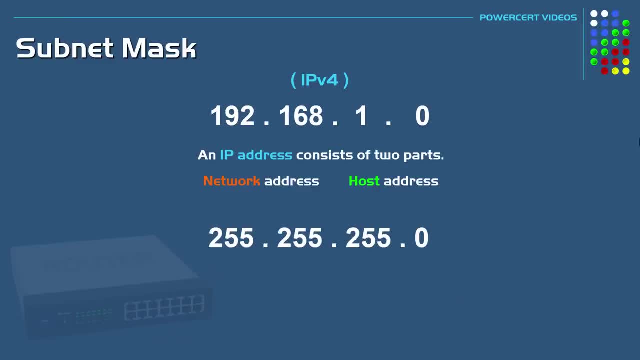 subnet mask comes in. A subnet mask is a number that resembles an IP address and it reveals how many bits in the IP address are unique. So an IP address is a number that is similar to an IP address and it reveals how many bits in the IP address are unique. A subnet mask is a number that is. 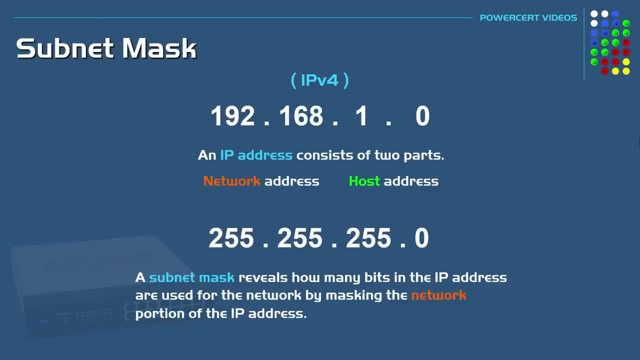 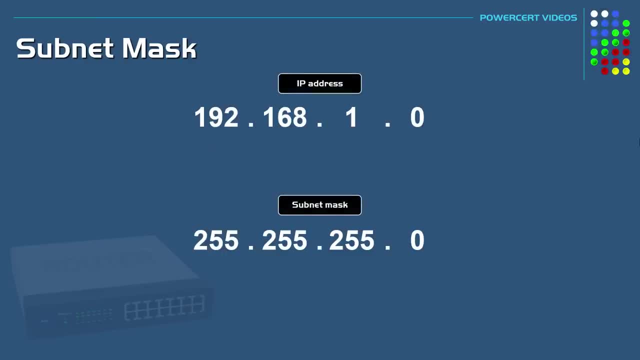 used for the network by masking the network portion of the IP address. Now, in the world of computers and networks, IP addresses and subnet masks in this decimal format here are meaningless, And this is because computers and networks don't read them in this format, And that's because they 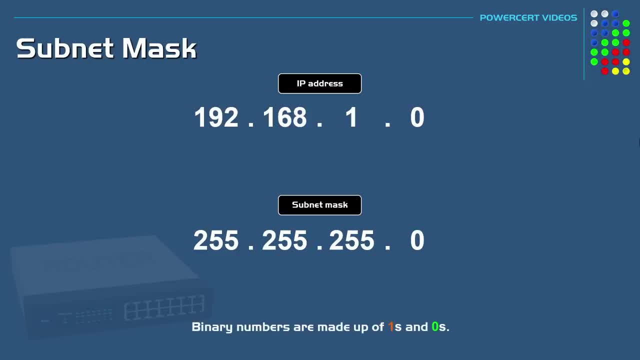 only understand numbers in a binary format, which are ones and zeros, And these are called bits. So the binary number for this IP address is this number here, And the binary number for this subnet mask is this number. And these are the numbers that computers and networks only understand. 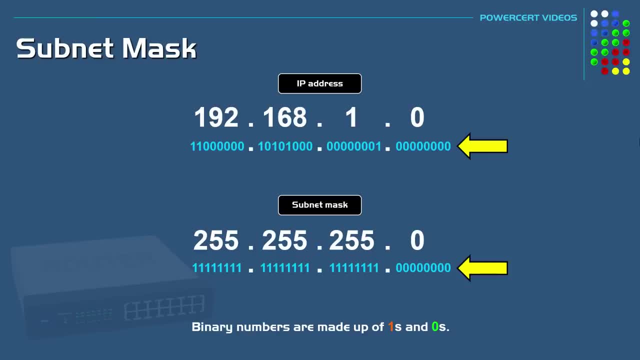 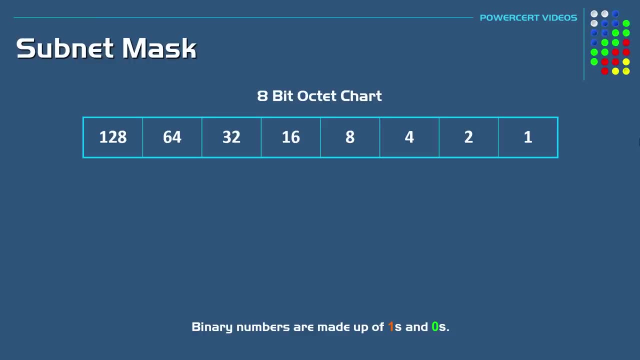 So the next question is: how do we get these binary numbers from this IP address and this subnet mask? So here we have an 8-bit octet chart. The bits in each octet are represented by a number. So, starting from the right, the first bit has a value of 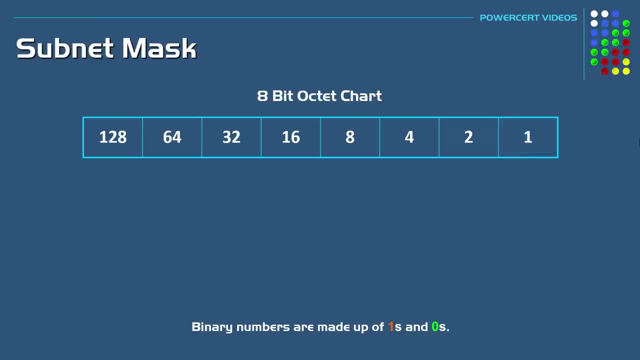 1. And then the number doubles with each step. So there's 2,, then 4,, 8, and so on all the way up to 128.. Each bit in the octet can be either a 1 or a 0.. If the number is a 1,, then the number that it. 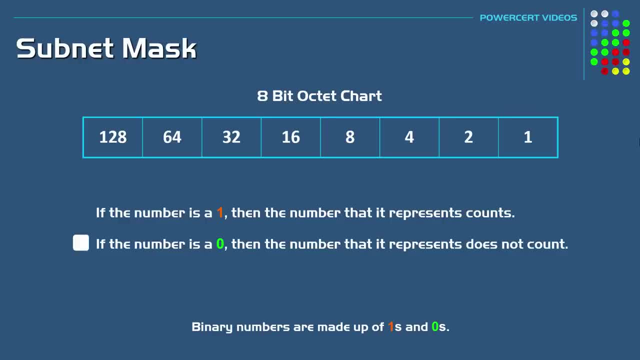 represents counts. If the number is a 0, then the number that it represents does not count. So by manipulating the ones and zeros in the octet you can come up with a number range from 0 to 255.. So, for example, the first octet in this IP address is 192.. So how do we get a binary number out of? 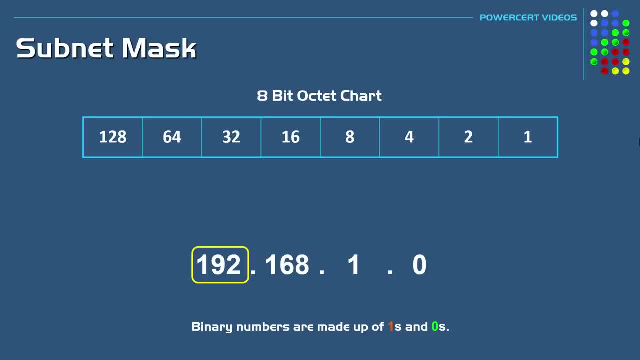 192?. First you look at the octet chart and then you will put ones under the numbers. that would add up to the total of 192.. So you would put a 1 in the 128 slot and then a 1 in the 64 slot. So 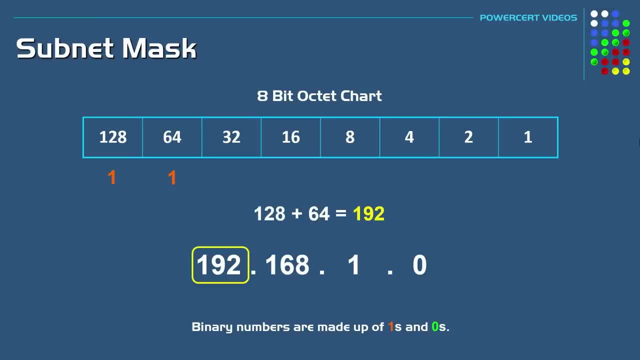 now, if we count all the numbers that we have ones underneath them, you would get a total of 192.. All the other bits would be zeros because we don't need to count them since we already have our number. So this number here is the binary bit version of 192.. So let's do the next octet. 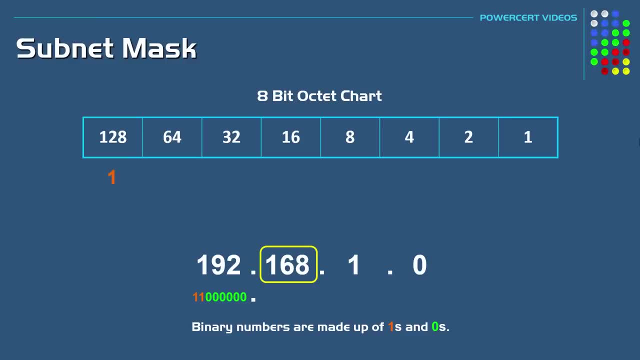 which is 168.. So let's put a 1 under 128,, 32, and 8. And then all the rest would be zeros. So if we were to add all the numbers that we have ones underneath them, we would get a total of 168.. 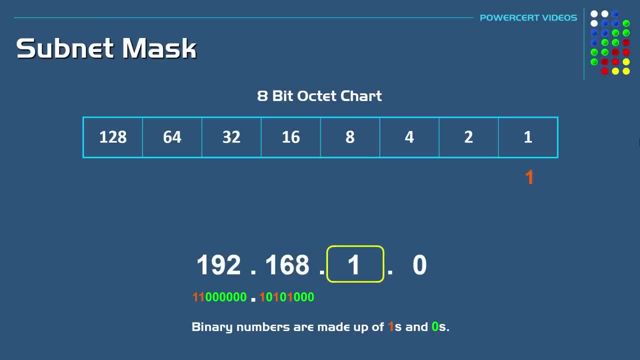 The next octet is 1.. So we'll put a 1 in the 1 slot and when you add up only 1, you get 1.. And the last octet is 0, which makes things simple, because all the binary numbers would be. 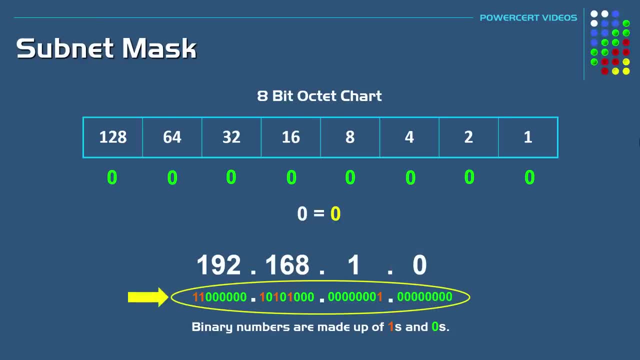 all zeros. So here is the binary number for our IP address. Now the subnet mask. binary conversion is exactly the same way. So in this subnet mask the first three octets are 255.. So if we were to look at this subnet mask in binary form, the first three octets would be all ones, because when you 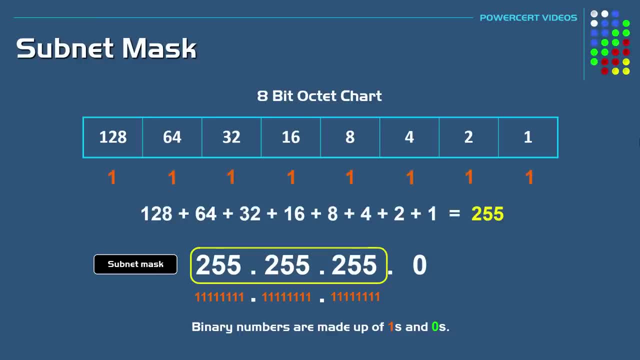 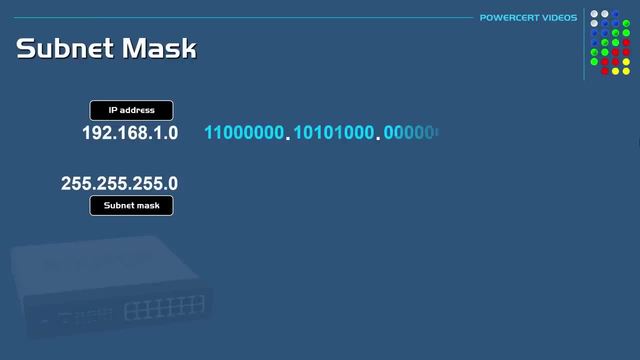 count all the numbers in an octet, it will equal 255.. And then the last octet would be all zeros. So here we have our IP address and subnet mask in binary form lined up together. So the way to tell which portion of this IP address is the network part is when the subnet mask binary digit. 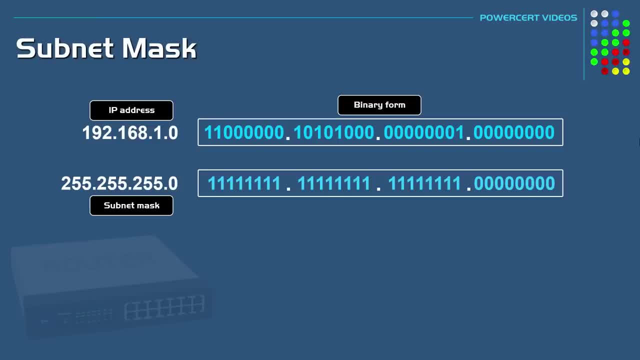 will indicate the position of the IP address that defines the network. So we'll cross out all the digits in the IP address that line up with the ones in the subnet mask, And when you do this it will reveal that the first three octets of the IP address is the network portion. 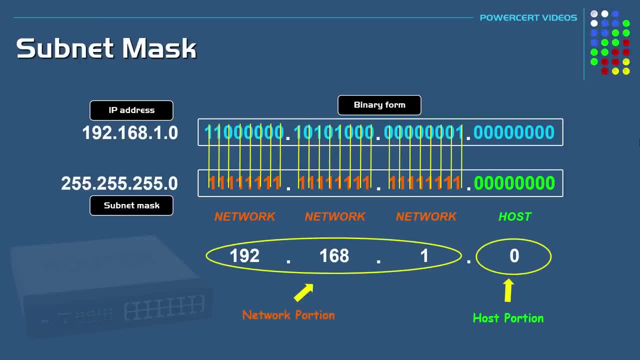 and the remaining is the host portion. So the ones in the subnet mask indicate the network address and the zeros indicate the host addresses. In another example let's use a different IP address and subnet mask and let's put them in binary form. So in this example the first two octets are 255,. 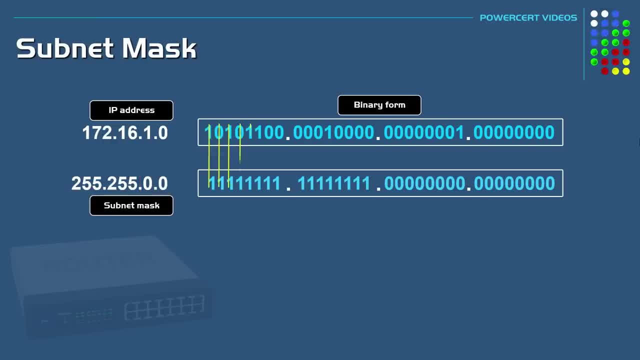 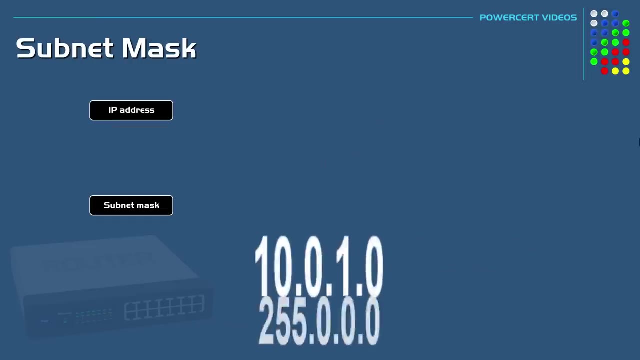 and the last two octets are zero. So if we cross out all the digits in the IP address that line up with the ones in the subnet mask, we'll see that the first two octets is the network portion and the last two octets is the host portion. And let's do one more. And in this subnet mask, 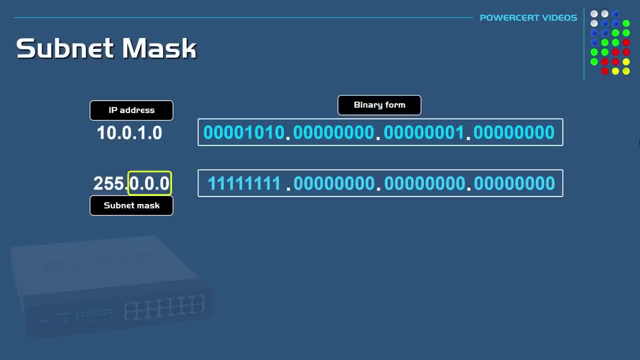 the first octet is 255, and the rest are zeros. And then we'll cross out all the digits again, and this time it reveals that the first octet is the network portion and the last three octets are for hosts. Now figuring out the network and host parts of an 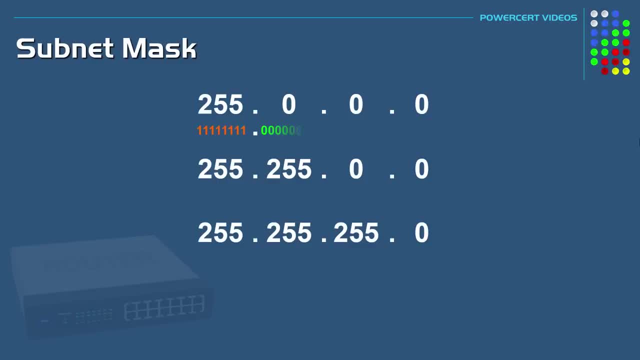 IP address. using these default subnet masks was simple Because, as I stated before, when you count all the numbers in an octet, it will equal 255.. So we automatically know that the numbers in the octet are all ones. So we really didn't have to see the IP address or 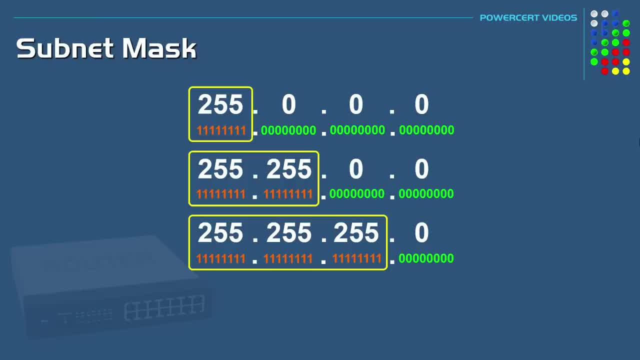 subnet mask in its binary format, because it's so simple. But what if the subnet mask was this number here, Where the first two octets are 255, but the third octet is 224. So this is a little trickier. So here is the binary number for this subnet mask. The first two octets are all ones. 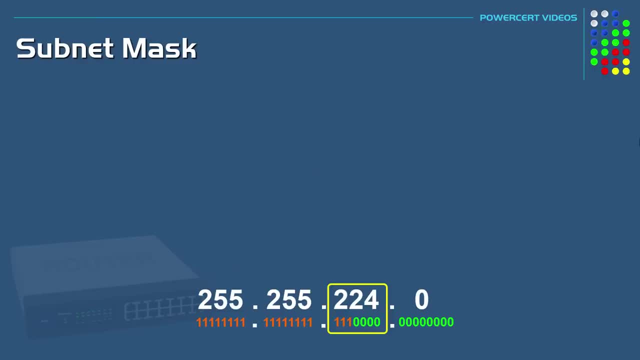 and in the third octet are ones which will equal 224, because, starting from the left, when you add the first three bits in an octet it adds up to 224.. So let's put this subnet mask and ip address in its binary format. 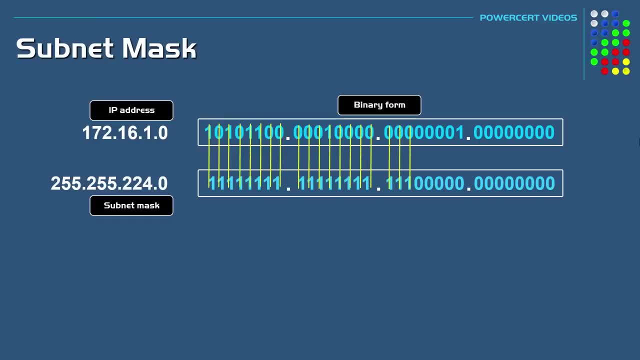 And again, if we cross out all the digits in the ip address that line up with the ones in the subnet mask, we'll see that in the ip address the first two octets and the first three bits in the third octet is the network part and the 13 remaining bits are used for hosts. So another question is: 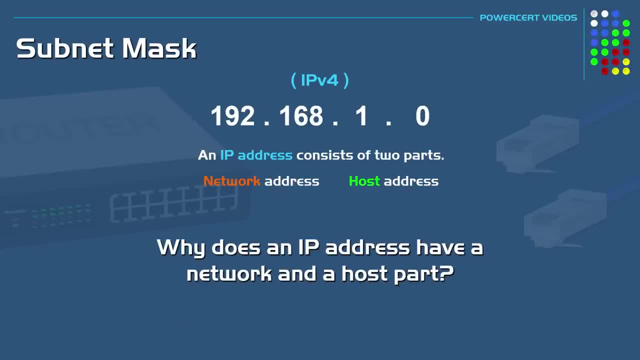 why does an ip address have a network and a host part? Why can't it just have a host part to uniquely assign each device an ip address? So why does it have a network part also? Now, the reason for this is manageability. It's for breaking down a large network into smaller networks, or 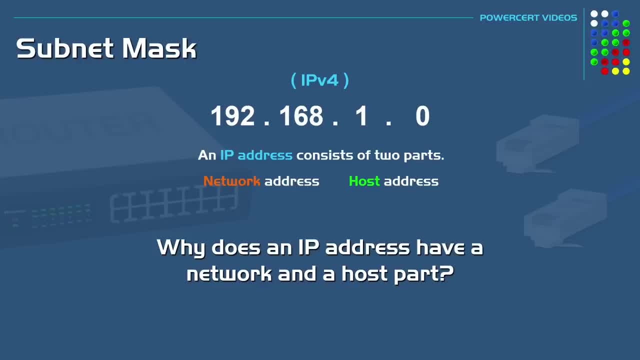 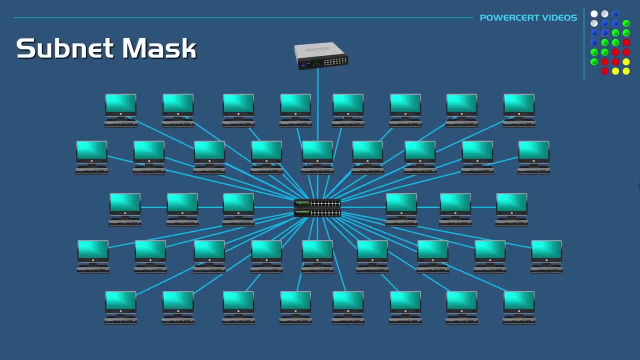 sub-networks, which is what we're going to talk about in this video. Now, the reason for this is known as subnetting. So, for example, let's say that there were no small networks. Let's say that an organization has a large amount of computers in one huge network. Now, when a computer wants to, 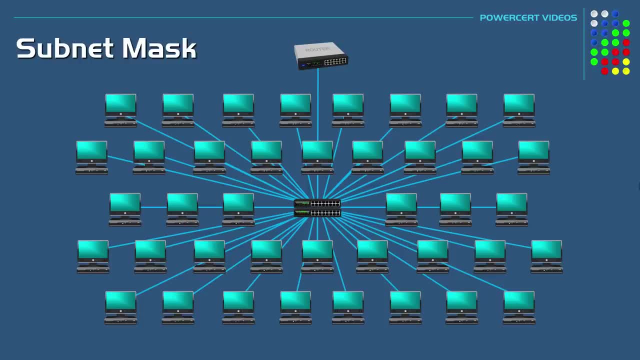 talk to another computer, it needs to know how and where to reach that computer, And it does this by using a broadcast. A broadcast is when a computer sends out data to all computers on a network so it can locate and talk to a certain computer. 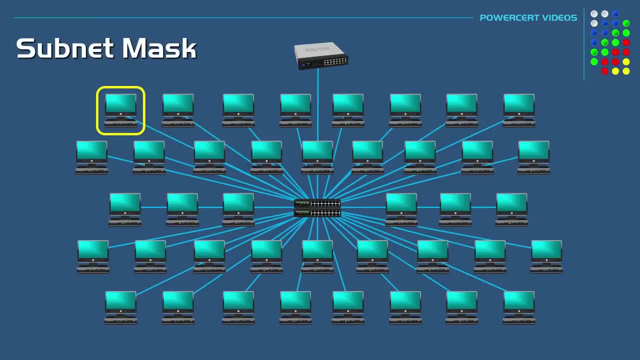 So, for example, let's say that this computer here wanted to communicate with this computer over here. So what happens next is that this computer here will send out a broadcast out on the network asking the target computer to identify itself so it can communicate with it. But the 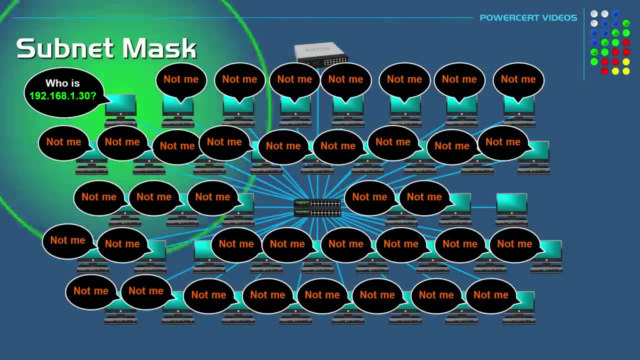 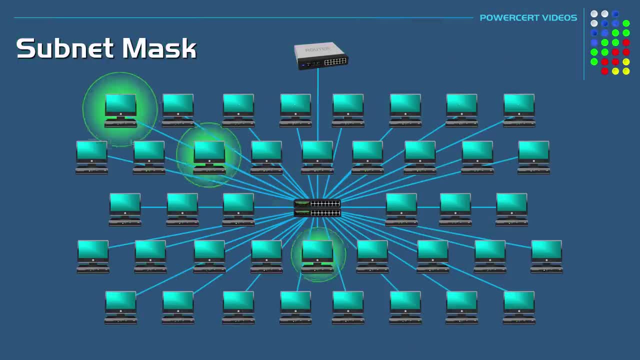 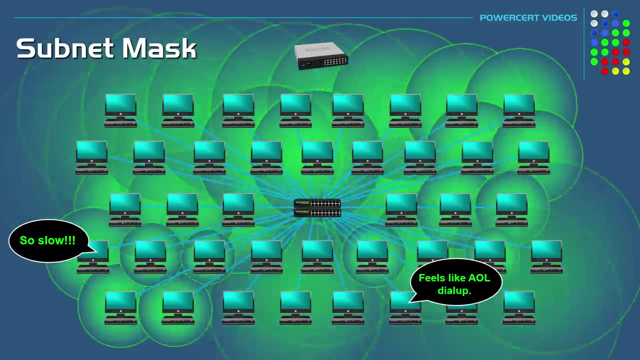 problem with this is that every computer on this network will also receive the broadcast because they are all on the same network. So, as you can imagine, if every computer on this large network was broadcasting to every other computer just to communicate, it would be chaos, It would. 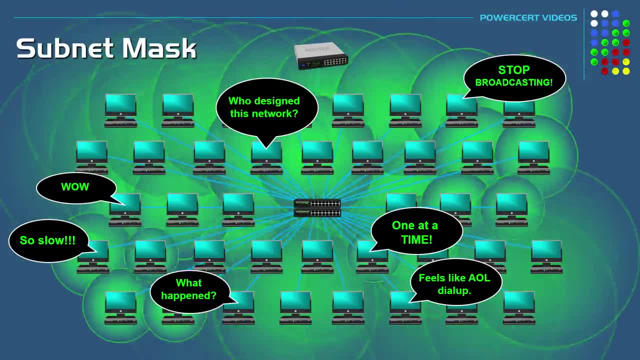 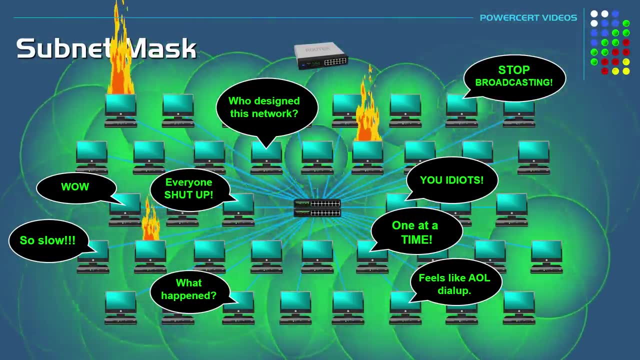 slow down the network and potentially bring it to a halt because of the tremendous amount of broadcast traffic it would cause, And it might even cause fires- Well, not really, but- And if a problem were to happen on the network, it would be very difficult to pinpoint. 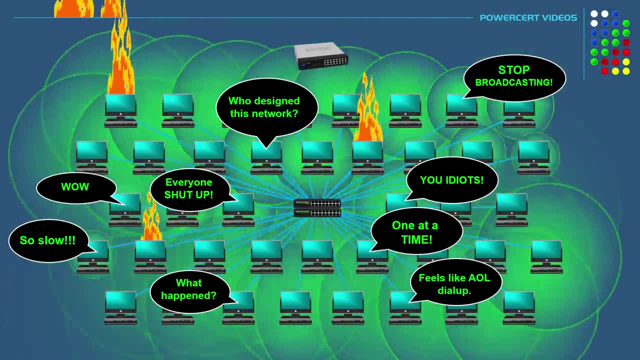 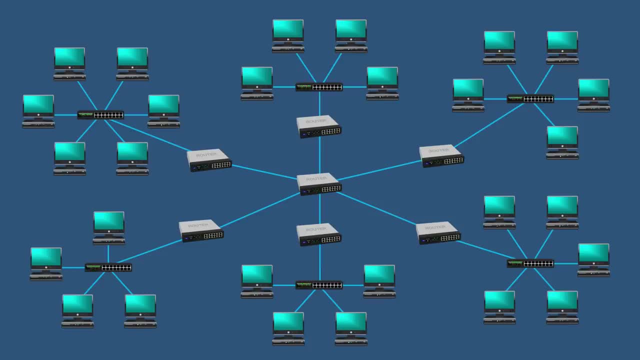 because the network is so big. So in order to prevent this, networks need to be broken down, networks And networks are broken down and physically separated by using routers. And by using routers, this would alleviate the problem of excessive traffic, because broadcasts do not go past routers. Broadcasts only stay within. 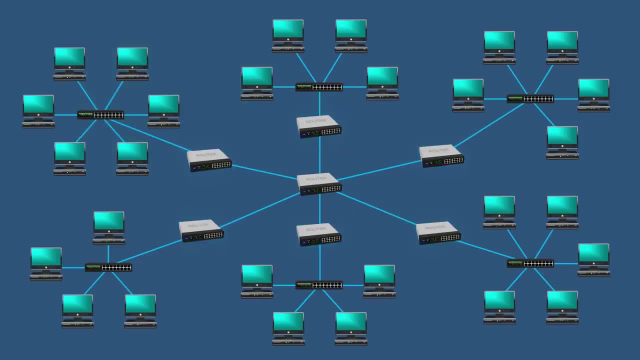 a network. So now, instead of one large network, this network is broken down into six sub networks or subnets. So now, if this computer here wanted to communicate with this computer over here, the computer will send out a broadcast that only the computers in its sub network can receive. But since the target 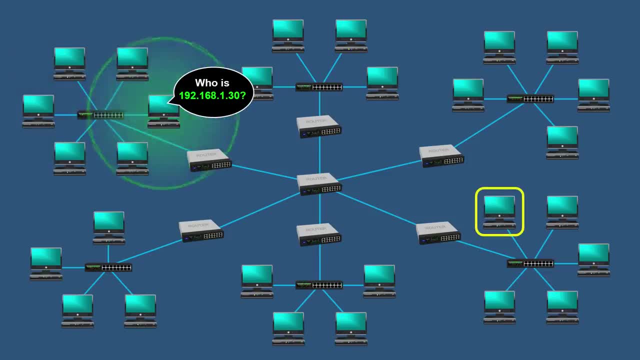 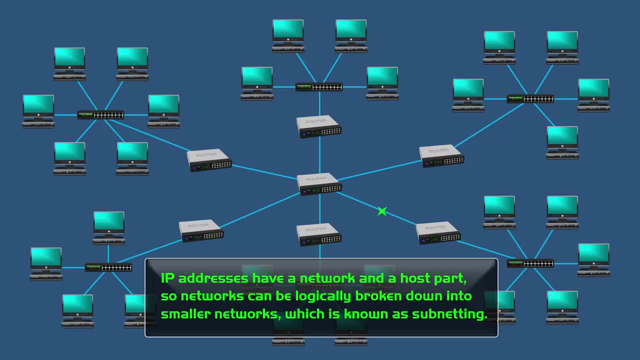 computer is on a different sub network. here the data will be sent to the default gateway, which is the router, and then the router will intelligently route the data to the destination. So this is why IP addresses have a network portion and a host portion, So networks can be logically broken down into smaller. 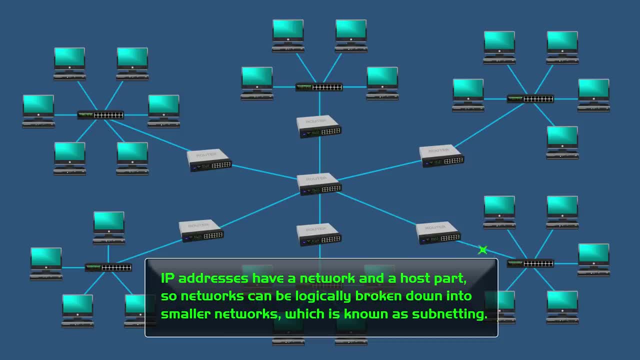 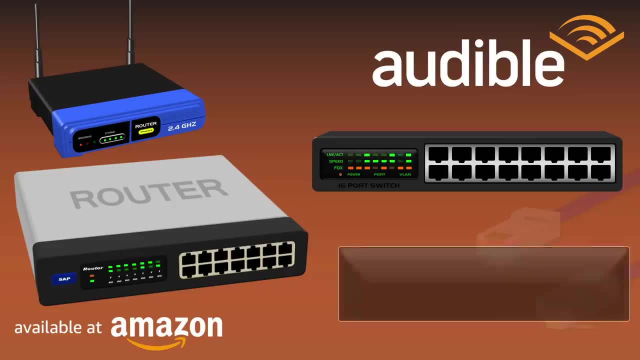 networks, Which is known as subnetting. Hey guys, I just want to break in here and tell you that if you're a beginner and you want to learn more about networking, I highly recommend an audiobook that will help you do that. I linked it in the 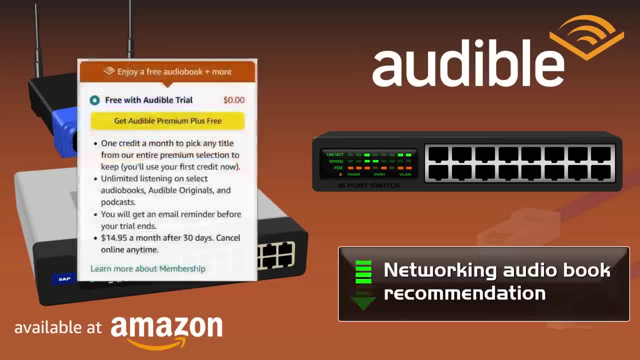 description below and you can download and listen to it for free. Just get the book by signing up for the free 30-day trial of Amazon Audible Premium Plus. But even if you cancel your Audible membership at any time during the 30 days, the audiobook is still yours to keep. 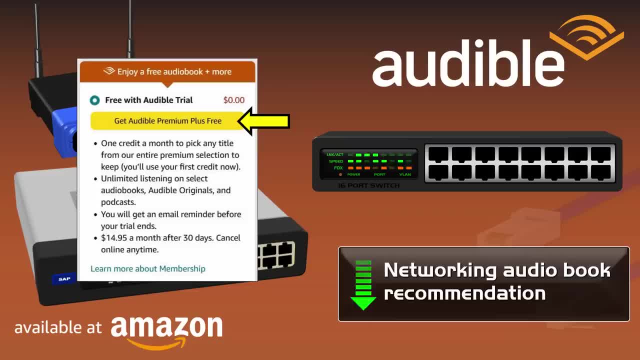 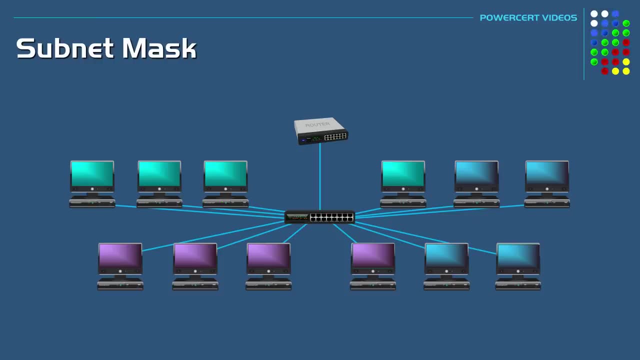 forever without paying anything. So just click the Amazon affiliate link below And by doing that, you'll also be supporting my channel, Because I still get commission even if you decide to cancel. So once again, it's completely free and thank you. So let's do an example here. So let's say that you have 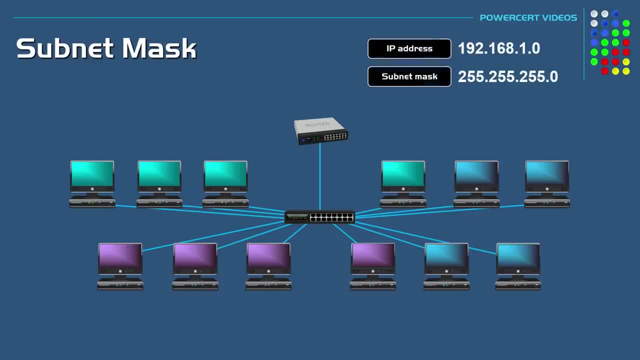 a small business and that this is your IP address and subnet mask. Now let's say that your small business has a total of 12 computers and all 12 of these computers are on a single network, And that's a lot of stuff, and that means that 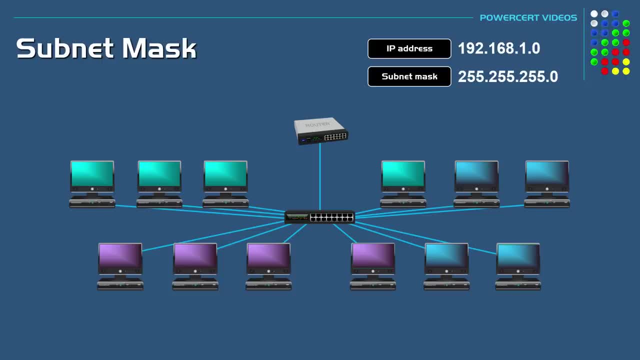 these computers belong to different departments indicated by their colors. But let's say that you wanted to separate the computers into three different networks so that each department won't see the other department's network traffic. So instead of having one network in your business, you want to break it down into three small networks. So the way to break this network down. 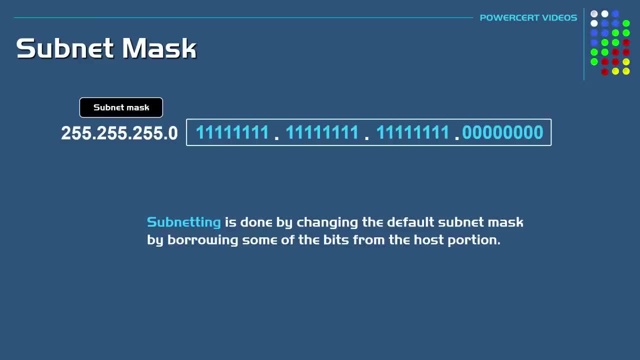 into smaller networks is by subnetting. Subnetting is done by changing the default subnet mask, by borrowing some of the bits that were designated for host and using them to create subnets. So in this subnet mask we're going to change some of the zeros in the host portion into ones. 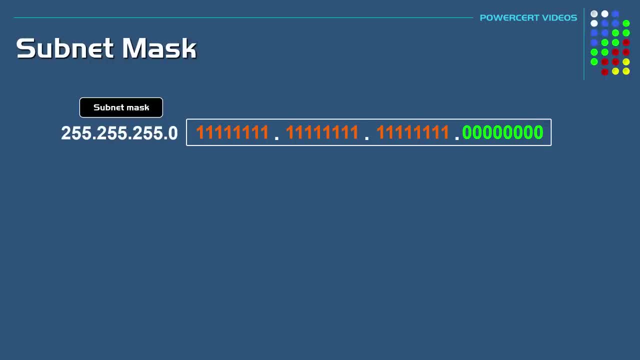 so we can create more networks. So if we leave the subnet mask the way it is, it will give us one network with 256 hosts. Now, technically we have to subtract two hosts because the values that are all ones and zeros are reserved for the broadcast and network activity. 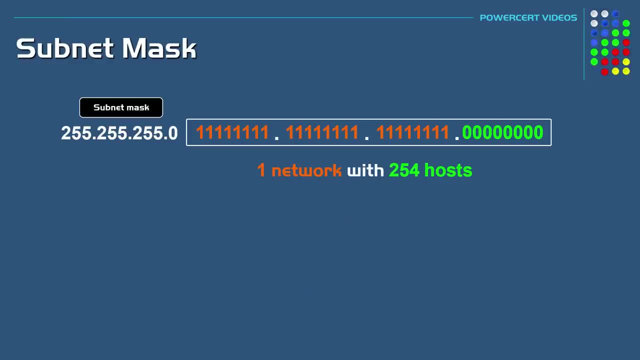 address respectively. So we actually have 254 usable hosts. But we need to change this subnet mask so we can produce the three networks that we need. So, for example, let's borrow one bit from the host portion. So here is our new subnet mask. So now the fourth octet is 128, because when you count, 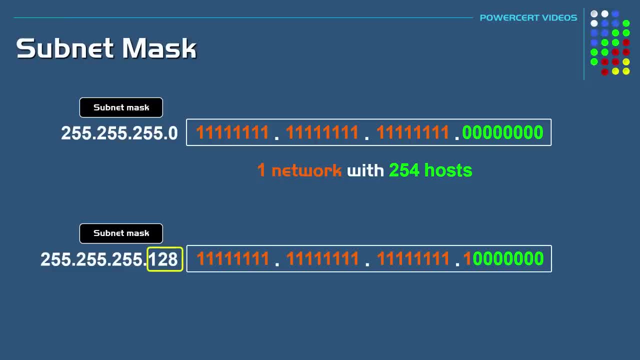 the first bit in an octet, it equals 128.. So by borrowing one bit, this will divide the network with 254 hosts. This will give us two networks, or subnets, with 126 hosts in each subnet. Now let's keep going and borrow another bit from the host portion, So now we are borrowing a total. 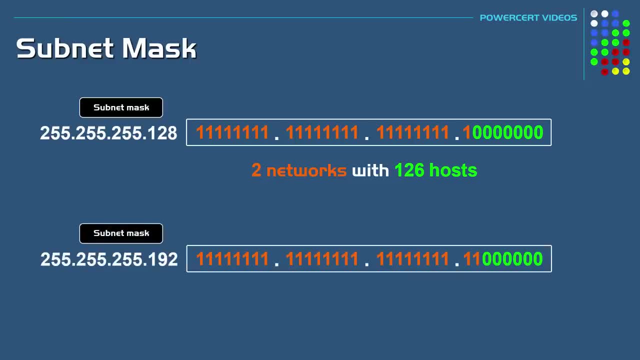 of two bits from the host portion. So here is our new subnet mask, and the fourth octet is 192.. So by borrowing two bits this will divide the network even further, and now it'll give us four subnets with 62 hosts each. 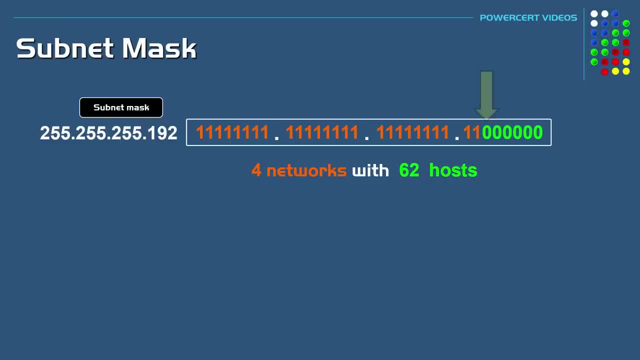 And again, let's borrow another bit from the host portion. So here is our new subnet mask and by borrowing three bits, this will divide the network into eight subnets with 30 hosts each. So if we continue breaking down this network, here is the result: if we borrow 4 bits, which will give 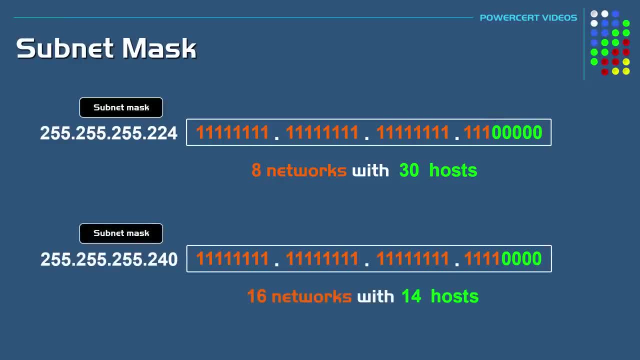 us 16 subnets with 14 hosts each. And here is the result: if we borrow 5 bits, which will give us 32 subnets with 6 hosts each, And if we borrow 6 bits, this will give us 64 subnets with 2 hosts. 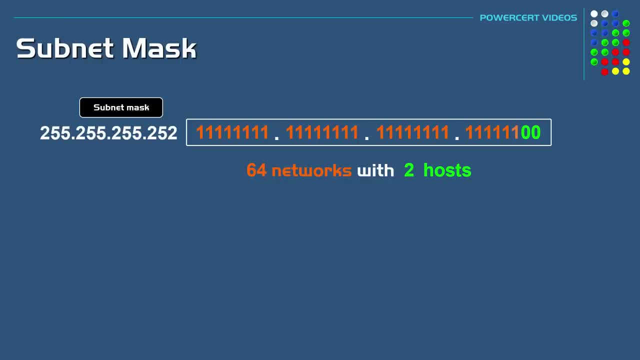 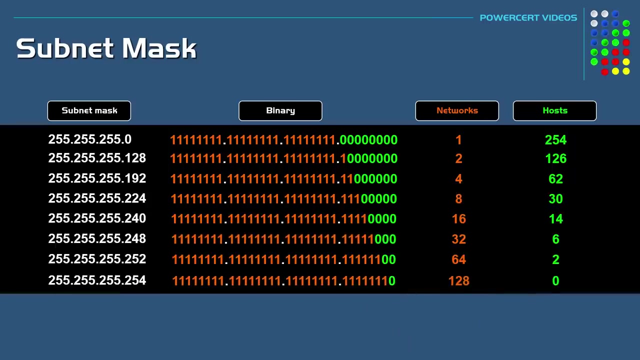 in each subnet. Now this is pretty much the limit, because if we borrow 7 bits, it will give us 128 subnets, but with 0 usable hosts. So, as you can see, the more bits the network portion borrows from the host portion, the amount of networks that can be created doubles with each bit. 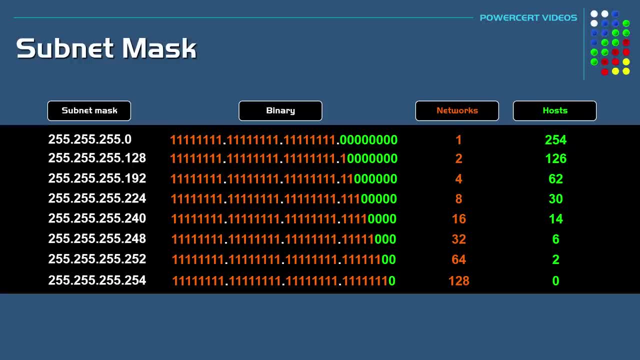 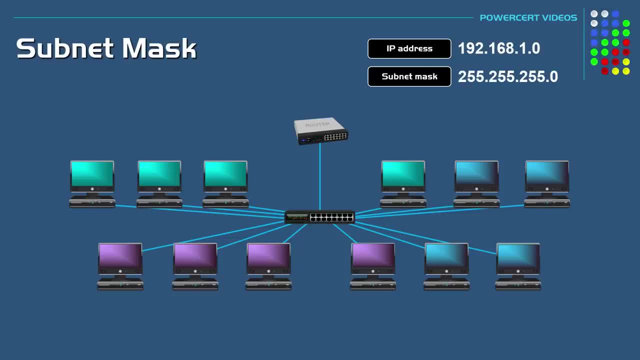 but also the amount of hosts per network gets cut in half with each bit. So, going back to our business example, if we wanted to break this network down into three smaller networks or subnets, we would have to borrow two bits from the host portion. So even though we only need 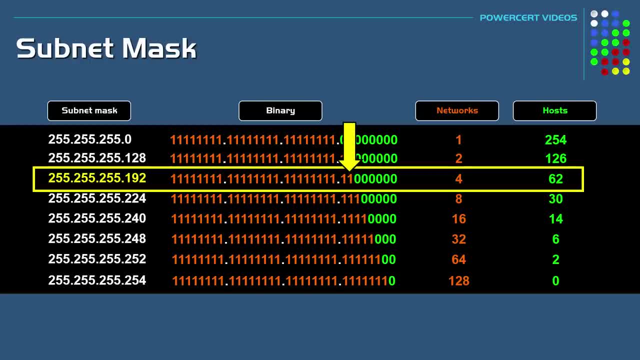 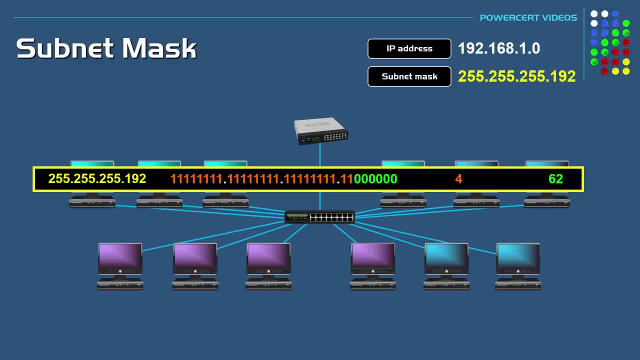 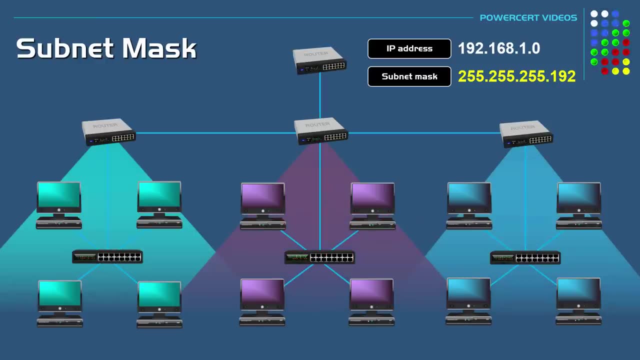 three networks. this subnet mask will give us at least four networks to work with. So our new custom subnet mask for our three subnets would be 255.255.255.1.. So now our network is broken down into three smaller networks or subnets. 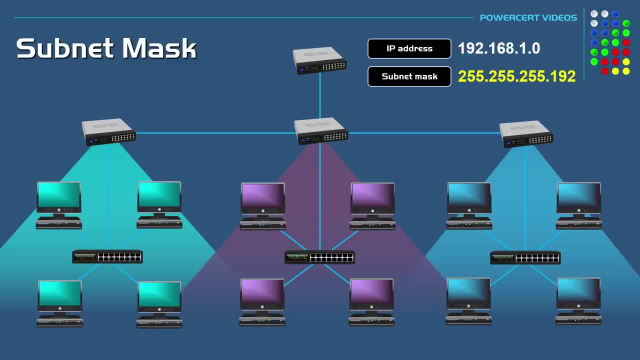 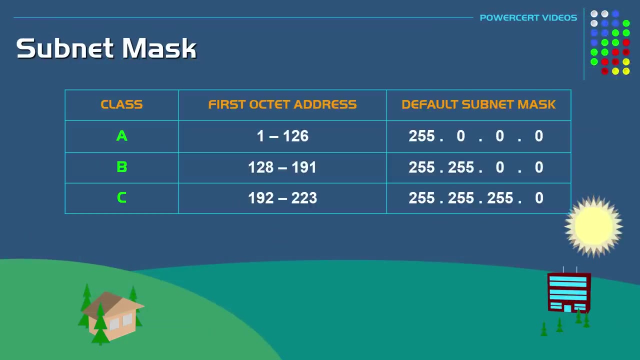 Now, just to be clear, this video is about subnet masks. This is not a full lesson on subnetting, because there's a little more to subnetting than what I showed you here. I'm just showing you how subnet masks relate to subnetting. Now IP addresses and subnet masks come in five different classes. 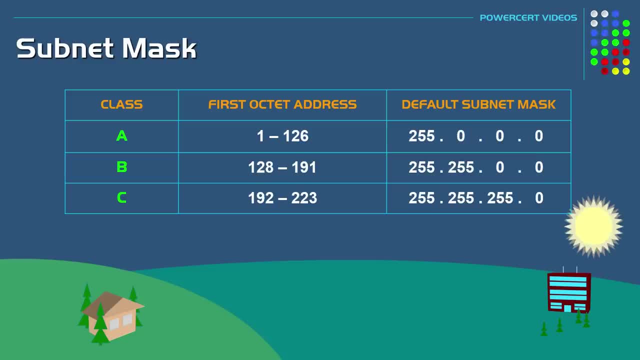 which are classes A through E. However, three of these classes are for commercial use. So here is a chart of the IP addresses and default subnet masks which are class A, B and C, And you can tell by the number in the first octet of the IP address and by the default subnet mask. 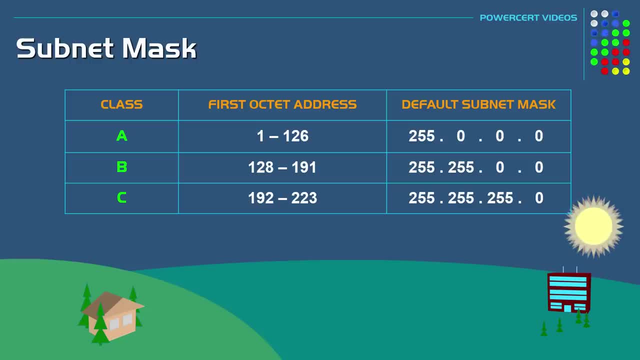 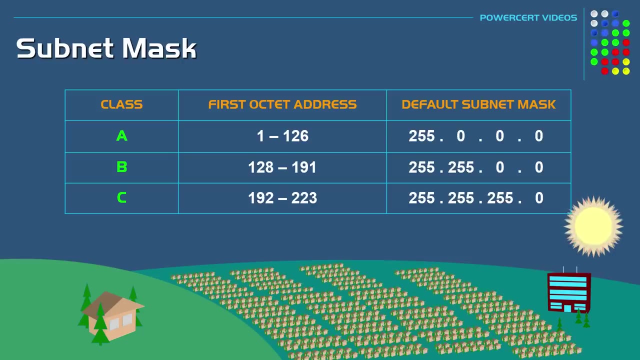 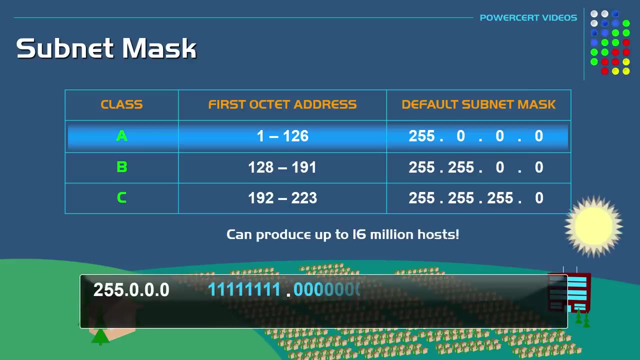 which class they belong to. Now, when an organization needs networking, they will need an IP address class according to the needs of that organization, which is based on how many hosts they have. So if an organization has a very large amount of hosts, they will need a class A IP address. A class A IP address can produce up to 16 million hosts.